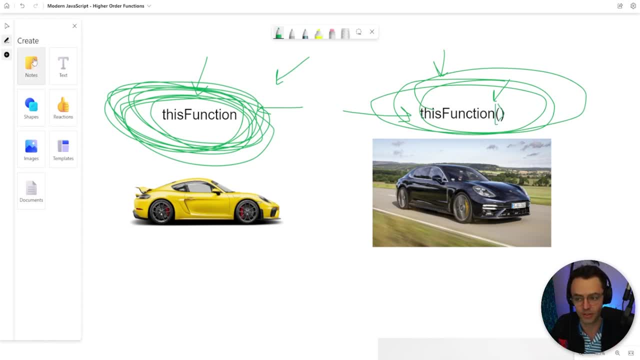 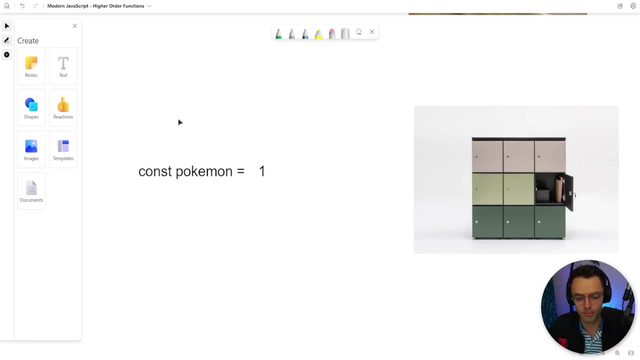 it will execute with the parentheses. So just keep that in mind, because that trips a lot of people People up. Another thing that is really confusing with people is that a lot of people can conceptually understand the fact that when we actually store a one in memory, it's just going. 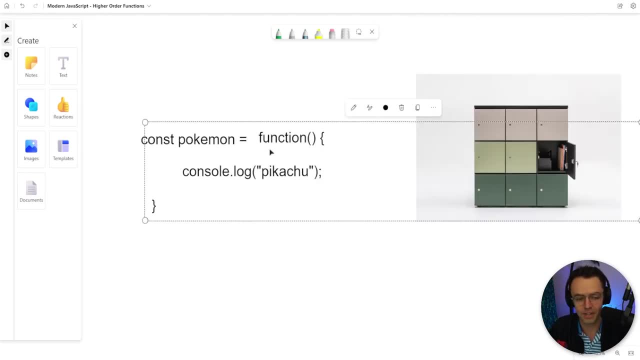 to be stored there. It's static, It's a one. But many times people can't understand how functions are stored in memory. And they are stored just like you store a one. A function is going to be stored in memory just like the one over here, And it's not going to be any different. The 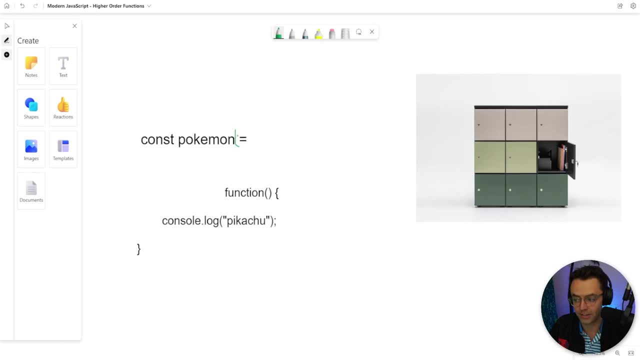 only difference is when you actually go to execute the function with the parentheses. Once you actually execute the function with the parentheses, it turns into an entirely different beast. Okay, So in this example up here, I have our previous Pokemon function that we were storing. 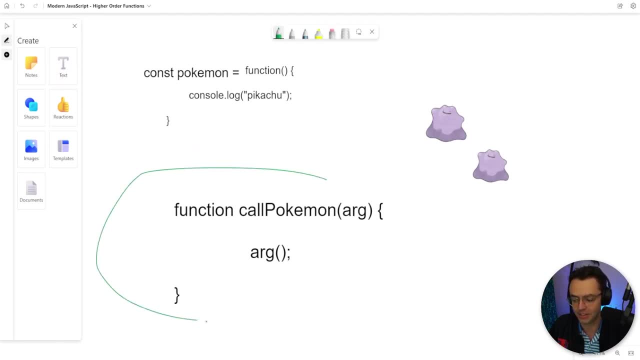 within the locker that we had before. This is an actual higher order function. This is an actual callback function. A callback function is a form of higher order function And this is a form of function, And it's going to be the one that you see 90% of the time. So we've talked about function. 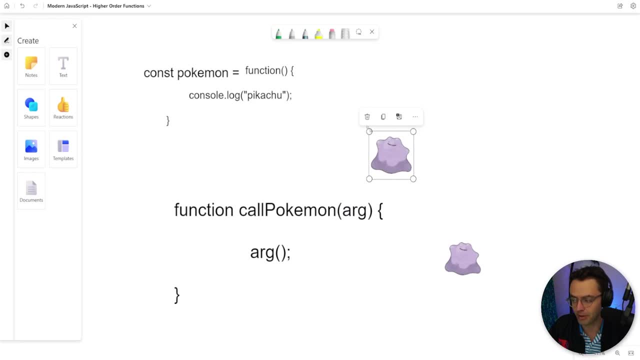 parameters. We have function parameters and our function parameters almost function like little dittos. Ditto is a Pokemon that changes shape into whatever you actually put inside of it. But callback functions are a little bit different. For the most part we're used to passing in strings. 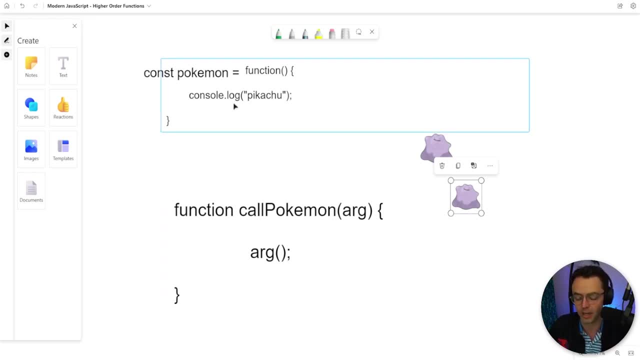 and numbers, And those are pretty easy to understand. But what a lot of people don't understand is what if you put a callback function in a function and it doesn't work? What if you passed in a function into another function? What if we actually passed in our Pokemon function up? 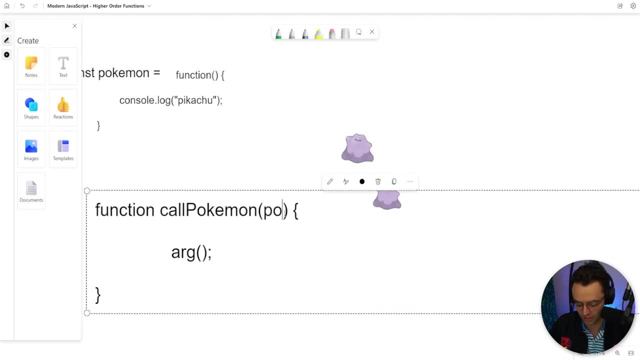 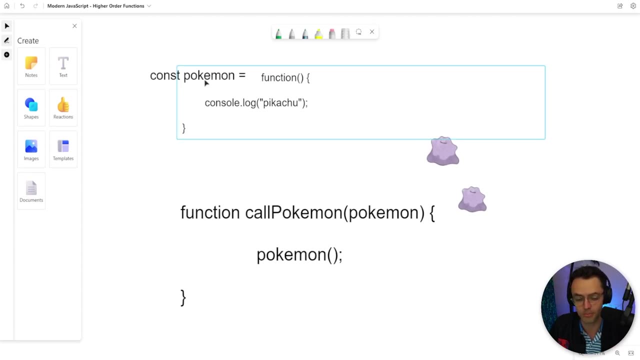 here And what would happen would be that it would literally change shape into the actual Pokemon And down here this part would execute as if this Pokemon function is executing right here. Now it's really important to understand that. What if we just passed in the Pokemon function right here? 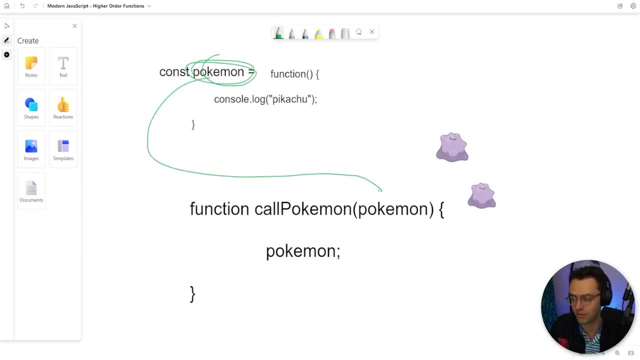 It would go into here. So this Pokemon is going to go down into our actual parameter right here, And then it's going to go down here When it's actually executed. it's an actual callback. At this point, right here, this function is not being executed. But 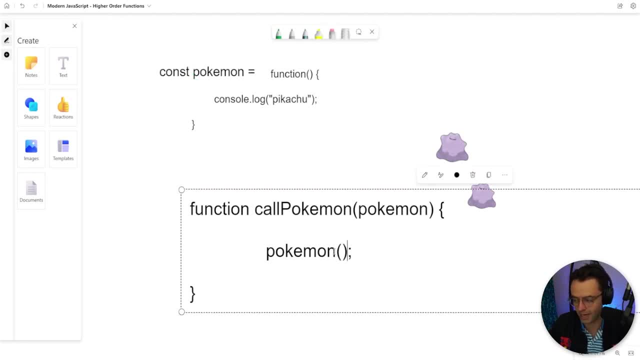 when we add the actual brackets right here, it will execute later on. So when we pass this function right down here, what's essentially going to happen is that this function is going to go down here And, instead of it being an arg, it's going to turn into the Pokemon function. that 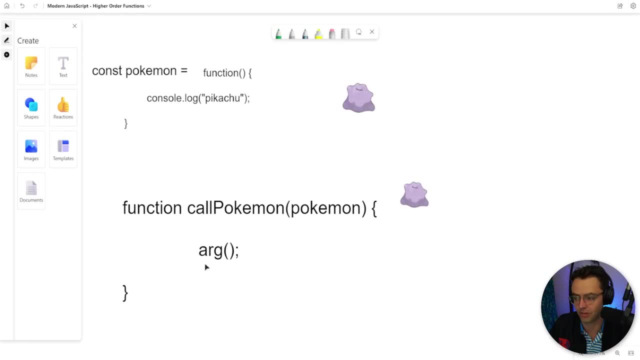 we had before, And then it is going to execute and just go down here, And then it's going to go down to this log, the console log that we had before, that simply just says Pikachu. So it's just going to change shape, similar to a Ditto, And it's going to execute that function inside the function, And 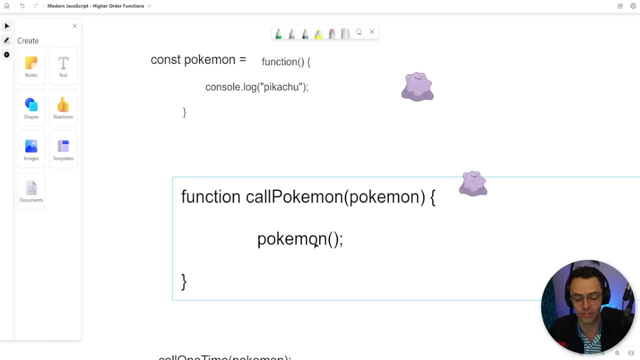 that is the whole entire idea behind higher order functions and callback functions. We'll talk about how functions return other functions here in a second. But this is just a good start until we can actually get our heads around how things actually work. So let's go inside Visual Studio. 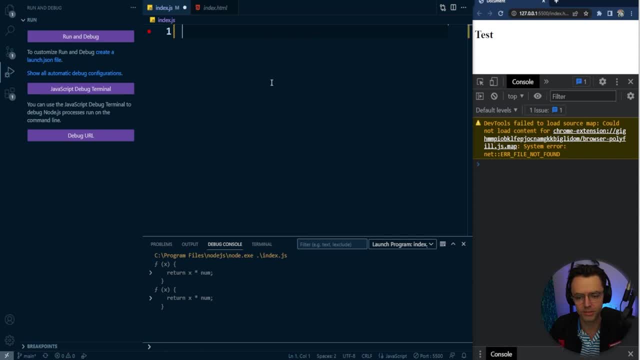 Code and let's actually practice. So let's go inside Visual Studio Code. Let's first start off by actually creating our callback function. So we're just going to here, I'm going to call this callback function And we are going to add a representative of the function that we plan to pass in, And then we will have three places. 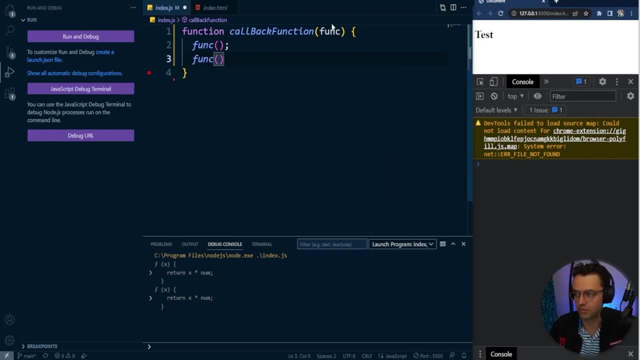 where we plan to execute this function. Just remember that this function that we are going to pass in is just going to go down here and it's going to execute. And it's going to execute because we have the parentheses And then we're going to have the 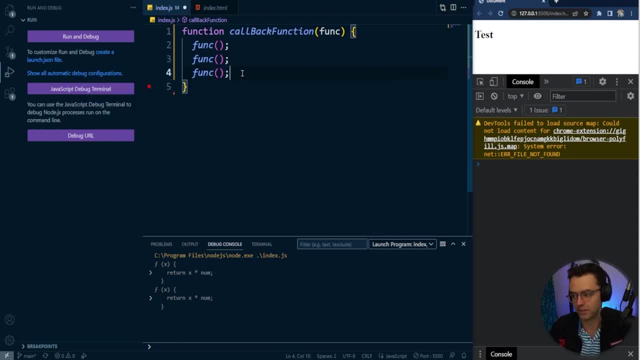 callback function. So let's just put another function down here, just like this, Very simple and easy to do. And let's just say we're talking about getting jacked, We're talking about steroids, Let's talk about some fighting. So what we're going to do is we're going to create a function about 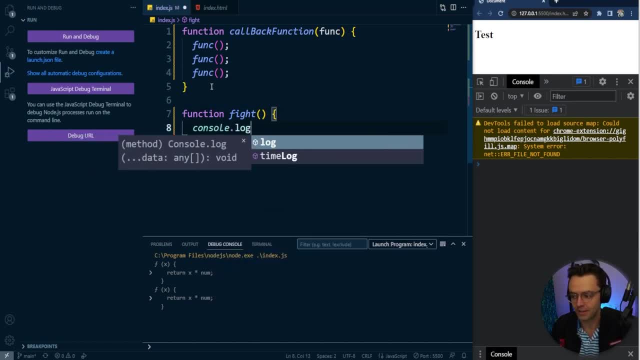 fighting And we're going to console log the type of rounds that we're going to throw. So we're going to go one, two, three Or no. let's just do a quick: one, two, one, two. We don't want to go. 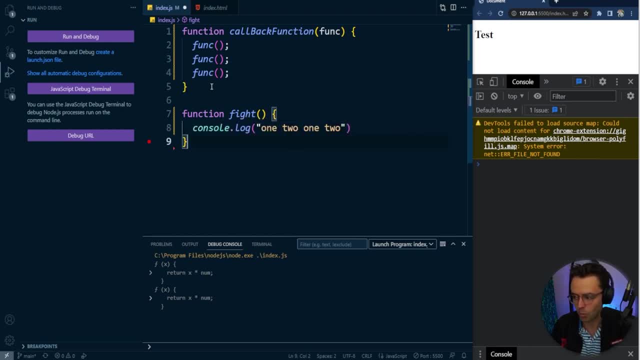 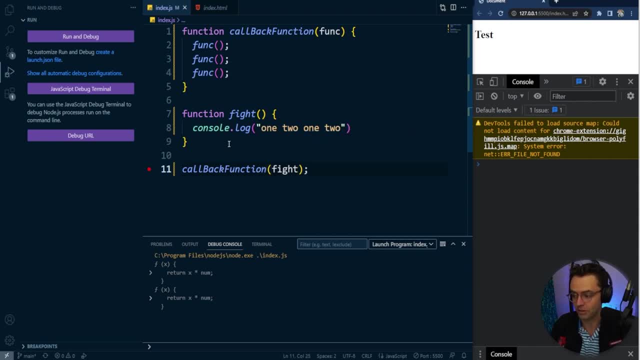 fight function into the actual callback function, where it is actually going to be executed. And I need to go in here and actually refresh my screen And, as you can see, it's being executed three times. So the function is going in, It's being passed in, It's going down here And it is indeed 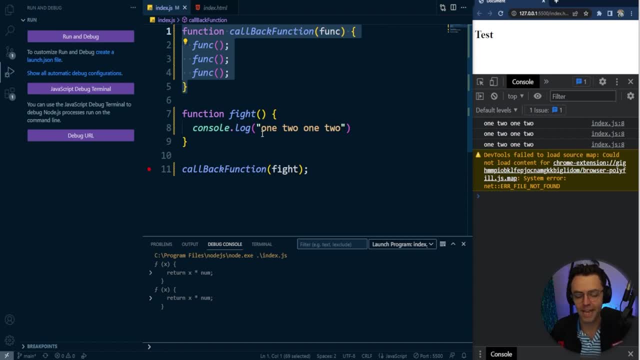 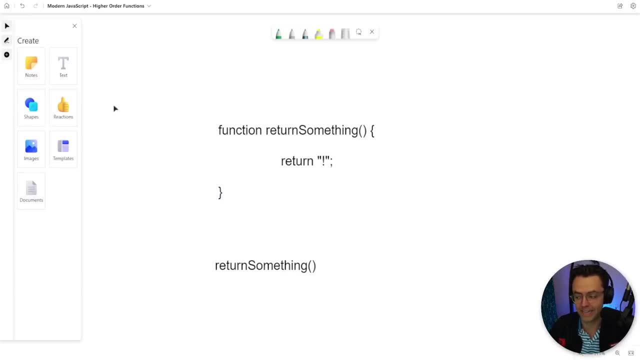 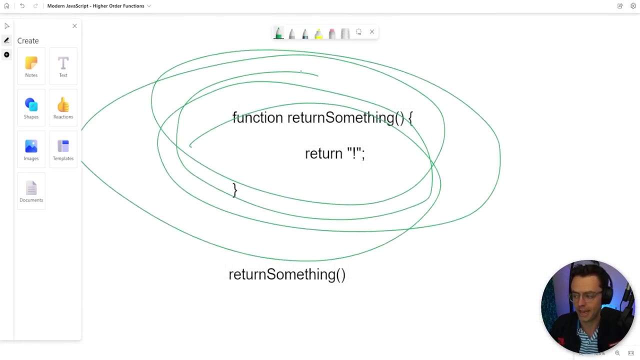 executing three times, But this is only half of the puzzle. The next thing that we need to talk about is how we actually return functions, And returning functions is not going to be that much more complicated. This is a regular function. This is probably what you're used to, And this is just 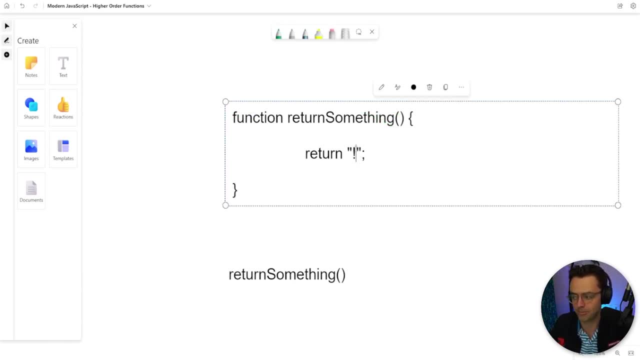 your run of the mill function And we're going to return an exclamation mark. But how would we take this function as boring, non-roided up function? We want our functions, you know, roided up. We want them looking good, And what we're going to do is we're going to do the same thing, but we're 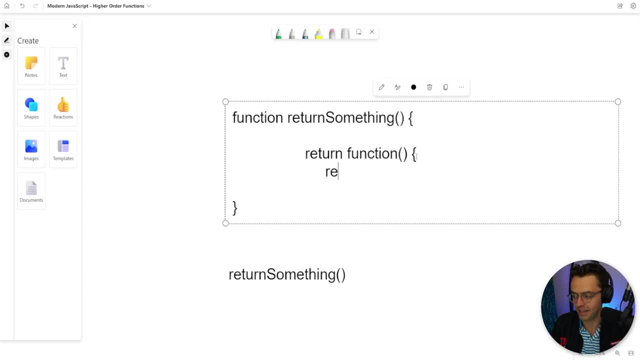 going to return a function that is not going to be executed. So we're going to return a function that just has the actual exclamation mark that we had before. Our previous function was a boring function, And what we did is we literally just took the function that we had before and put it. 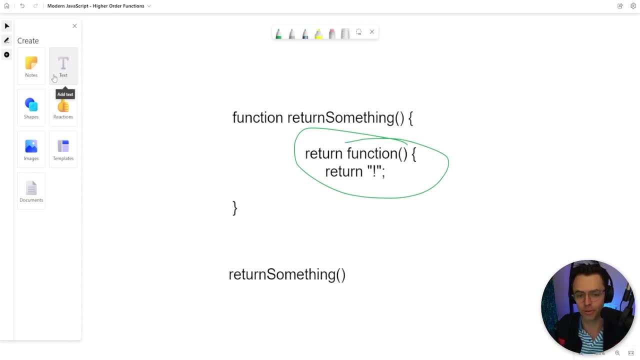 inside. Here's probably the most important part of the video. Like not joking, If you paid attention up until now, I guarantee you that you're going to be in a lot better place than people who just skipped the video. The way that you execute the inner function: you just put another set of 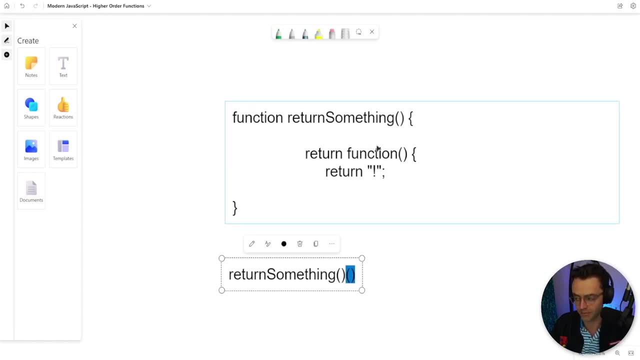 parentheses. If you want this function to execute the inner function as well as the outer function, you need to put the second parentheses And a lot of times you will see something along the lines of people just having result like this: and they execute the first function, So it'd be return. 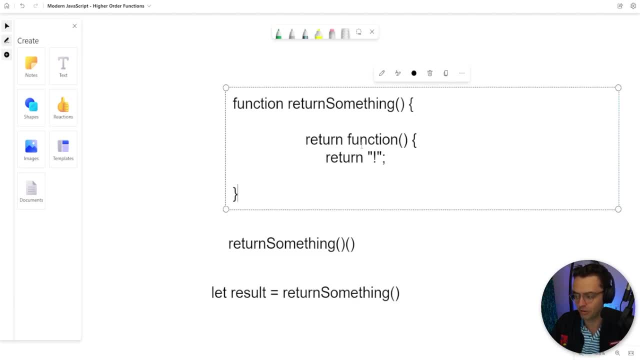 something And what's going to happen is is that it's going to return this function. So this part right here is going to actually go inside of this part right here, And then this is when you're going to actually want to console log or do whatever you want You can put it. 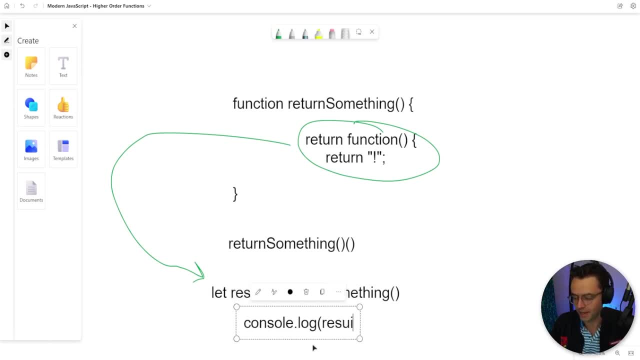 somewhere else or put it into another variable, but I'm just going to actually execute it. This is the part when you take the result and then you execute it again, And this is when it's going to execute the inner function. So you can do it either way. You could do it this way, which is not usually as.